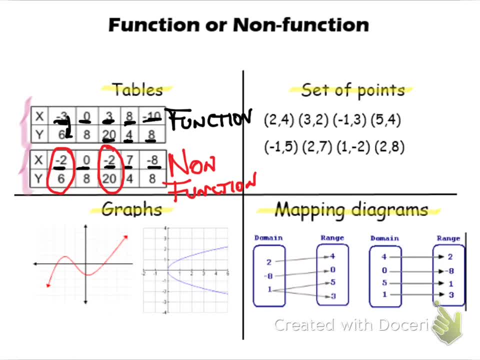 Now looking at our set of points. I look at the first one and notice that I have the x values of 2,, 3,, negative 1, and 5.. None of my x values are repeated, So I can assure that this will be a function, because there's no way I will get different y values for the same y. 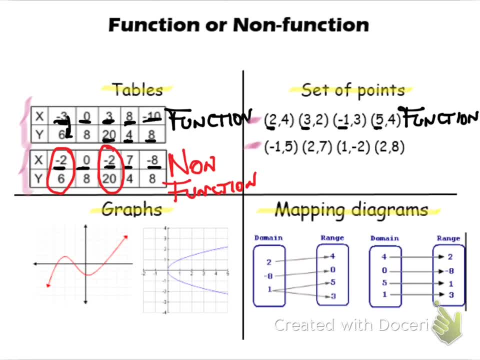 Now, if I look at my second list of set of points, I will notice that my x values are negative: 1,, 2,, 1, and 2.. So notice how we have the negative, the value of 2, twice paired with different y values. 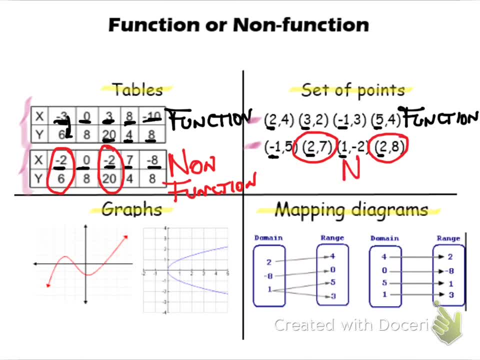 So the same x is given to me, Giving me different y's. That will be a non-function When we're talking about graphs. we're going to look at our first graph And we're going to check this a little bit different. 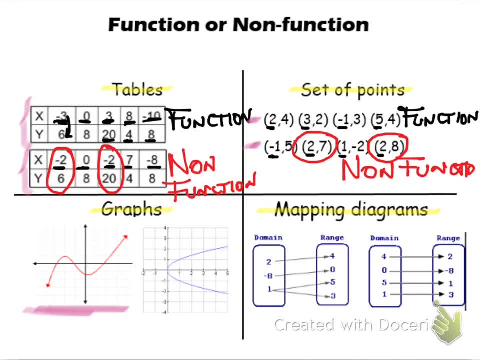 We are going to do what is called the vertical line test, And that is, imagine a set of different vertical lines passing through the line And the rule is they could only touch your line once. So, for example, this one only touches my y here. 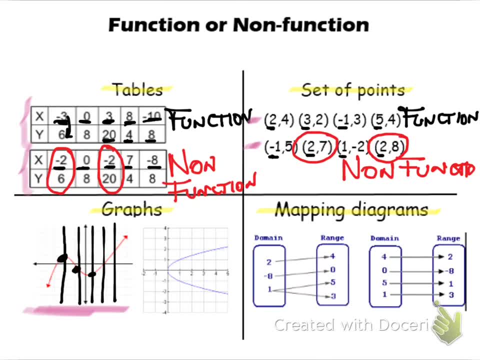 This one touches the line only here, only here and only here. So each one of my lines is touching the vertical lines are touching the line only once, So that will be called a function. Now, if we look at our second graph, 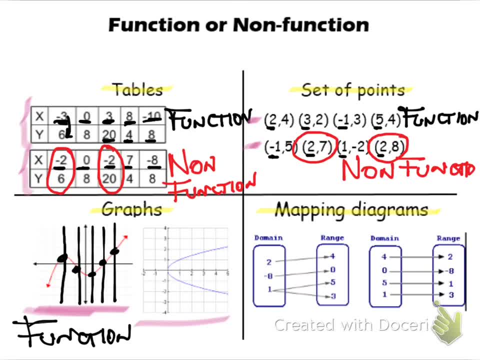 We will notice that if I start drawing my vertical lines, I immediately notice that the same line, the same vertical line, will touch twice. That immediately tells me that this is a non-function. It's a non-function For mapping diagrams. I'm going to use my same definition. 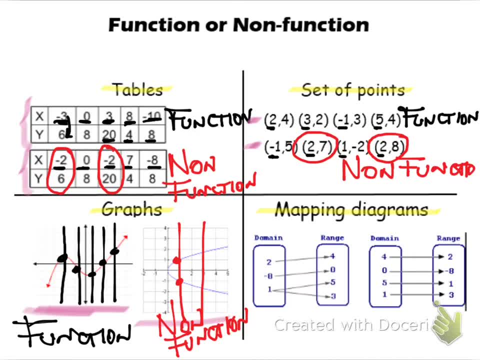 Every x cannot have only one y value. So I want you to look exactly at the value of negative one. in the first mapping diagram It's paired with two different y values, which is five and three. That will tell me that this is a non-function. 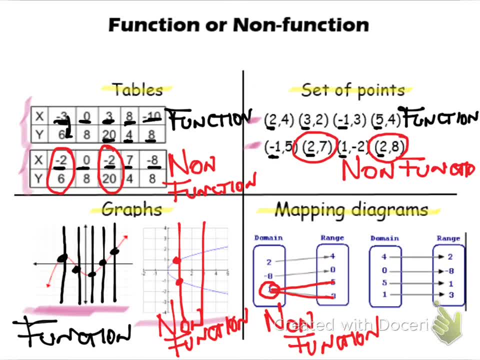 And in our last mapping diagrams you can see how each x value is paired only with one y value. That will tell you that this is a function.